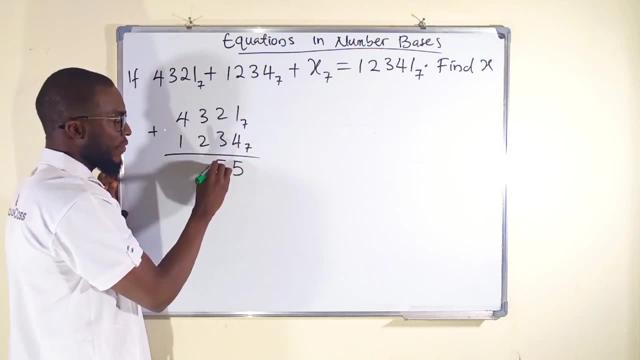 But 5 is less than the base. 2 plus 3 is also 5.. 3 plus 2 is 5.. 4 plus 1 is also 5.. This is base 7.. Now this is the solution After adding these two numbers together. 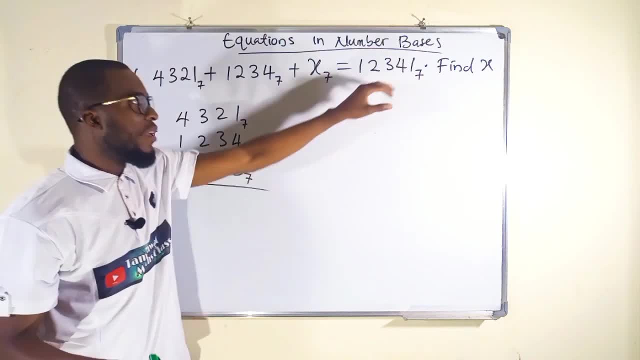 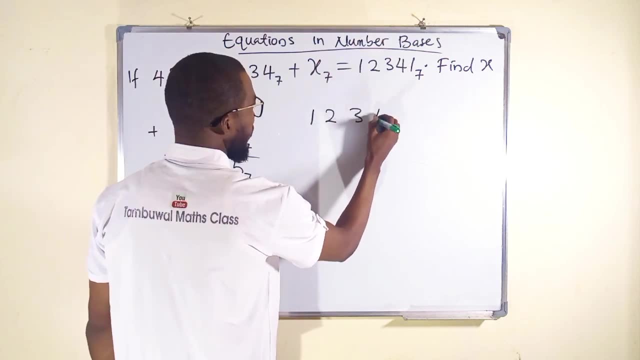 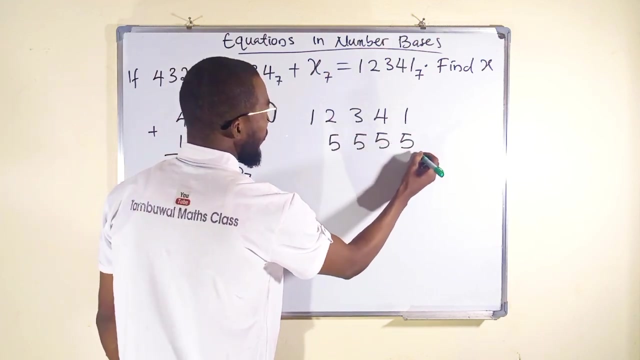 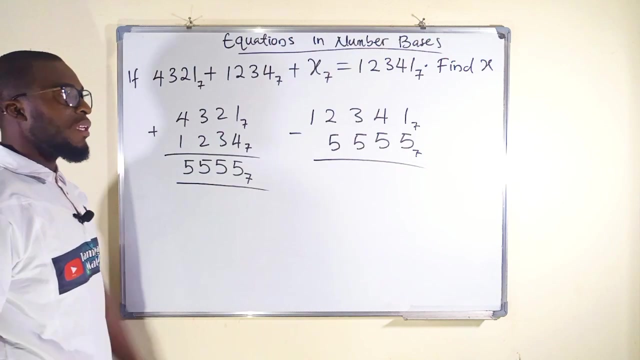 To find x. we are going to remove this 555 into here. So we say 12,341 minus 5, 5, 5, 5.. All these numbers are base 7. We are now subtracting. Whatever we obtain is the value of this unknown. 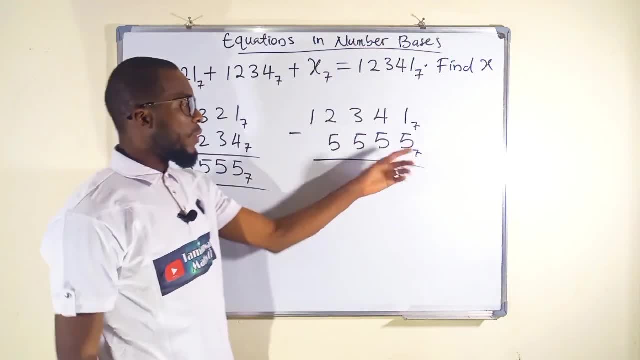 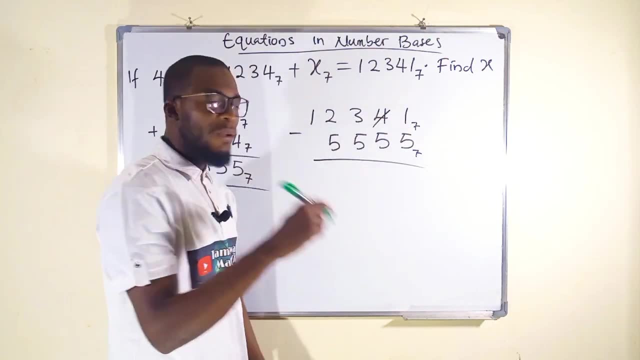 1 minus 5,. you know, definitely it cannot happen, Unless if you want to get a negative result, And hence we are going to borrow here. This is 4 bundles. Remove a single bundle, You will be left with 3 bundles. 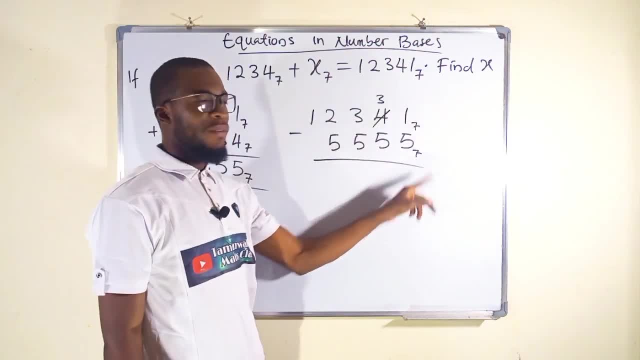 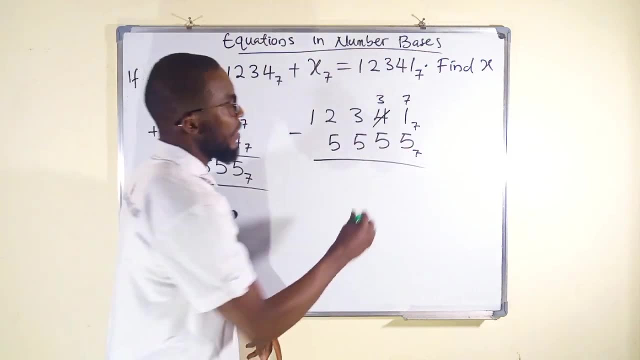 What is coming here is exactly equal to the base 7.. You bring it as 7.. You join it with this one, it becomes 8. Then that 8 minus 5, you know- is 3. We have 3 here. 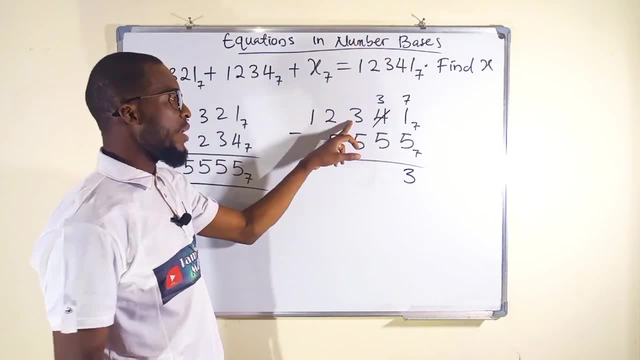 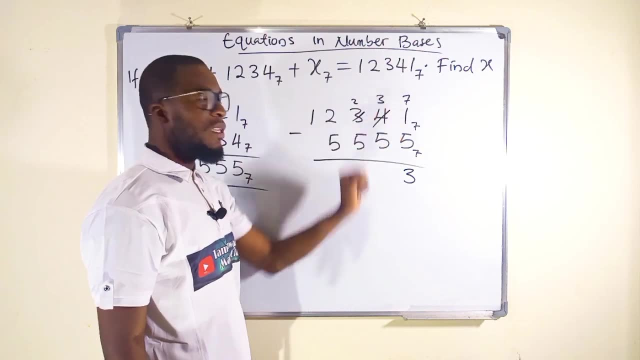 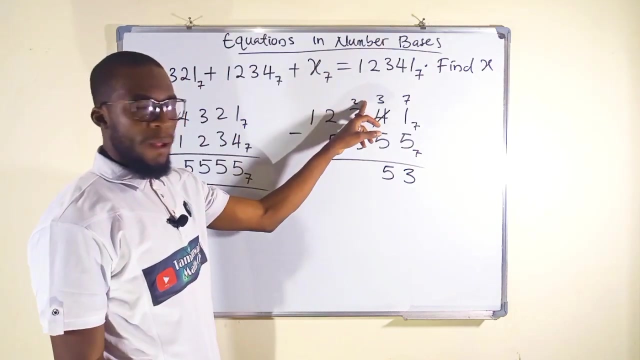 It cannot subtract 5, unless we borrow here: Taking away one bundle here, leaving 2.. Bringing it here as 7 plus 3, will make it 10. And 10 minus 5 is 5.. We have 2 here. 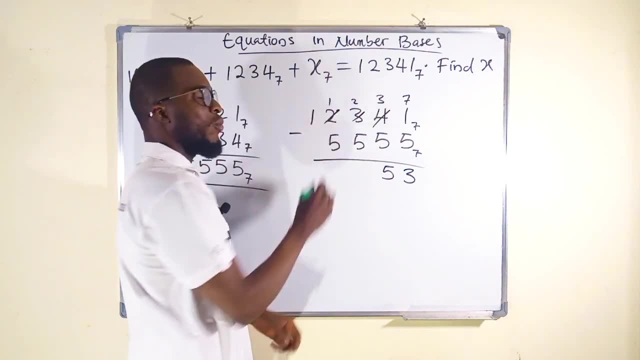 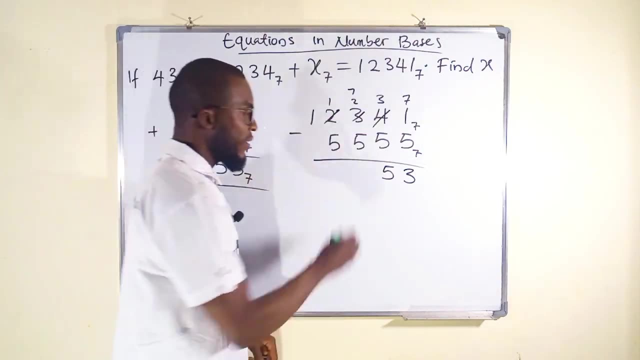 It cannot subtract 5.. We take away one bundle here, leaving 1. We bring it here as 7.. Then 7 plus 2 is 9. Then that 9 minus 5 is 4. We have one bundle here which cannot subtract 5.. 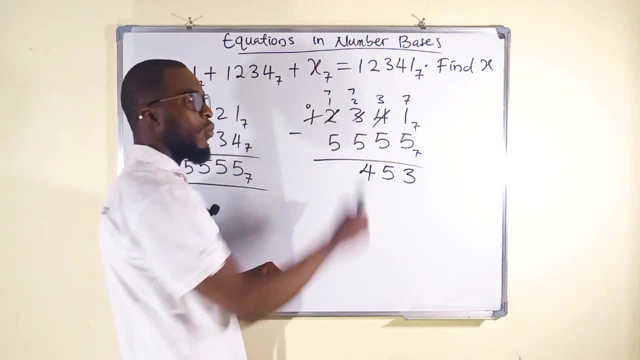 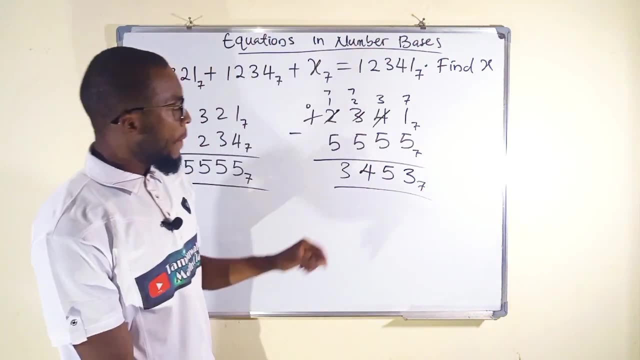 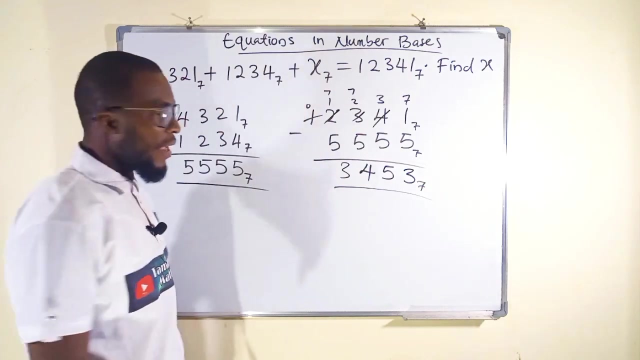 We take away this bundle, leaving nothing. We bring it here as 7 plus 1 is 8.. Then 8 minus 5 is 3. In base 7.. So 3453 is equal to this x. So finally we see x equal to 3,, 4,, 5.. 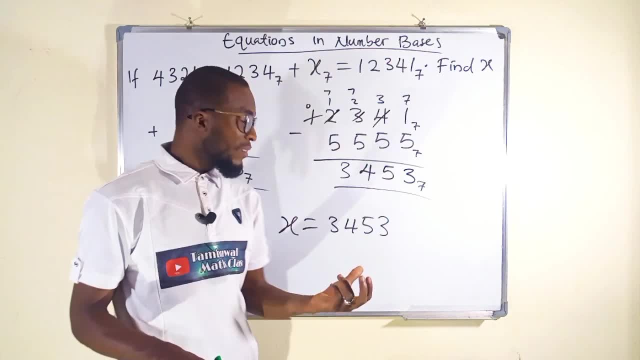 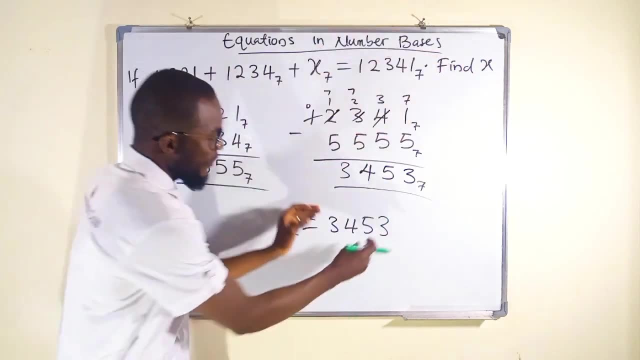 3. On the standard, a question. I always say it is: have the answer, do not include the base. Look at, x is already in base 7.. The question says: find that x. So if you take this value, you replace it here. it will meet the base there. 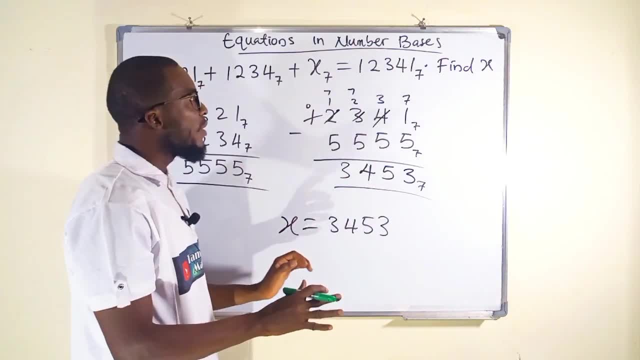 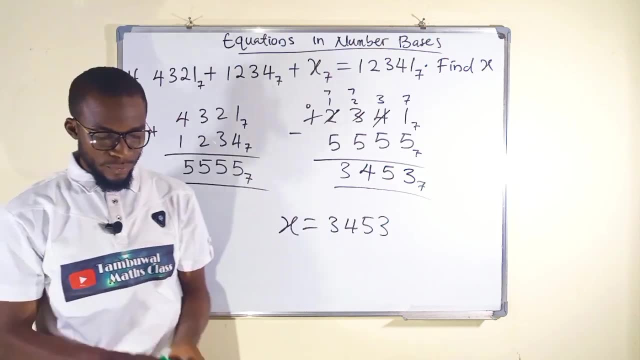 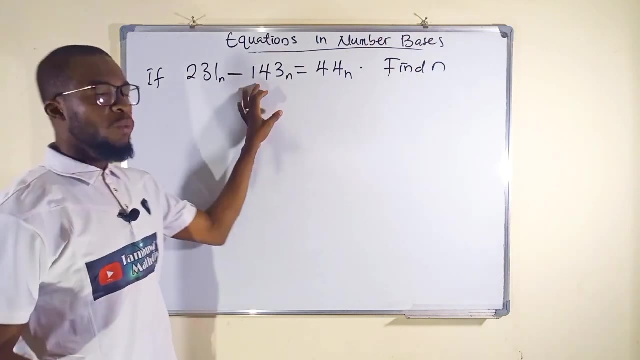 We are not asked to find x in particular base, We are only asked to find that x. So this is the value. Now let us look on to the next question. So here is our second question. It says: If 231 in base n minus 143 in base n equal to 44 in base n, what is this base n? 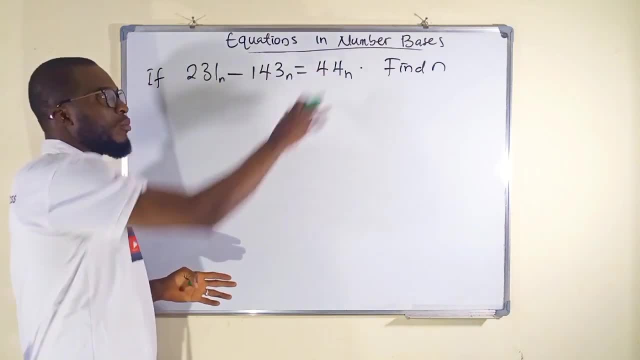 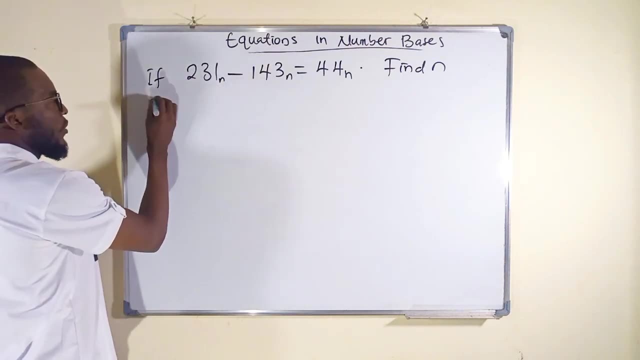 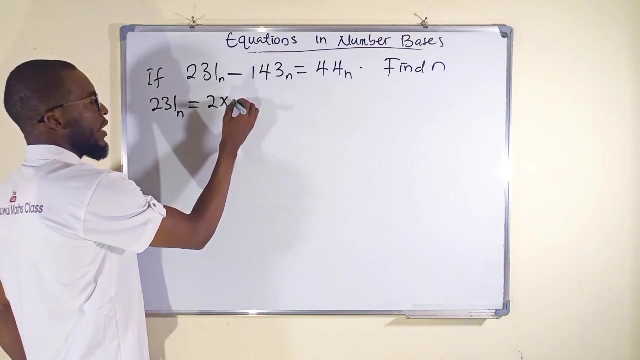 Since we don't know the base n, we can convert each of these numbers into base 10.. So to convert this into base 10, we say 2,, 3, 1 base n will be equal to 2 times the base n. 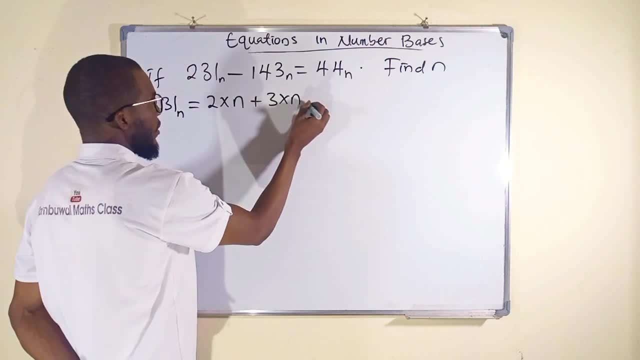 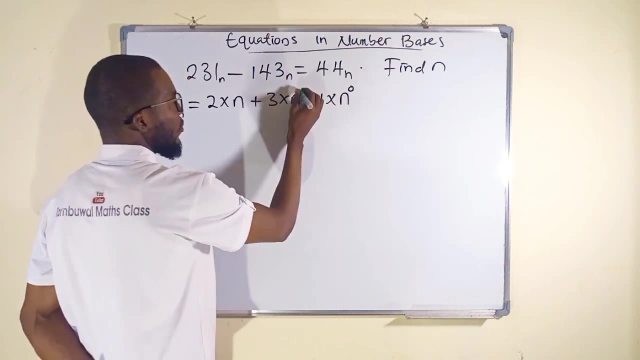 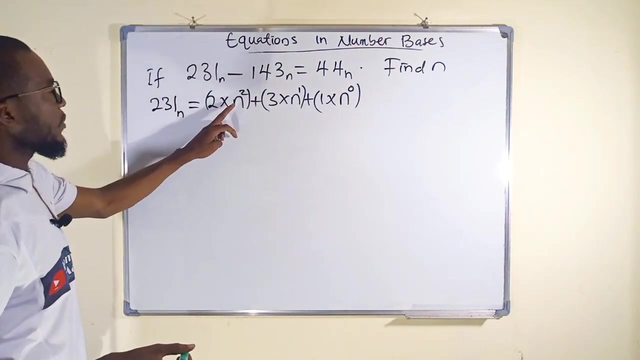 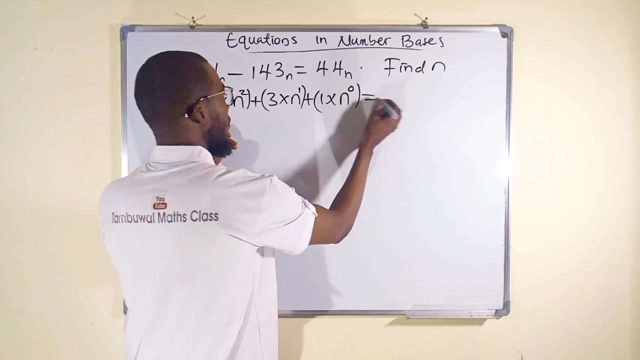 Plus 3 times the base, plus 1 times the base, You assign index 0,, 1 and 2.. n power 2 is still n power. 2 times 2 will give us 2 n power 2.. n power 1 is n power 2.. 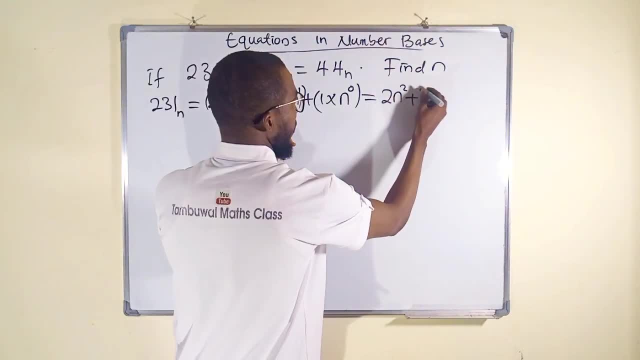 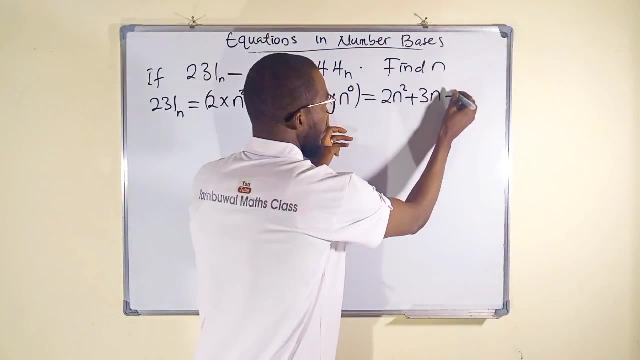 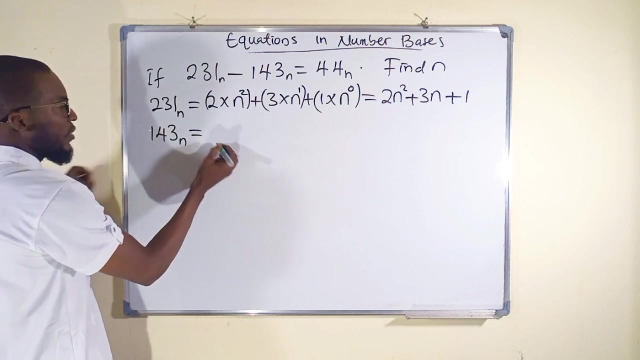 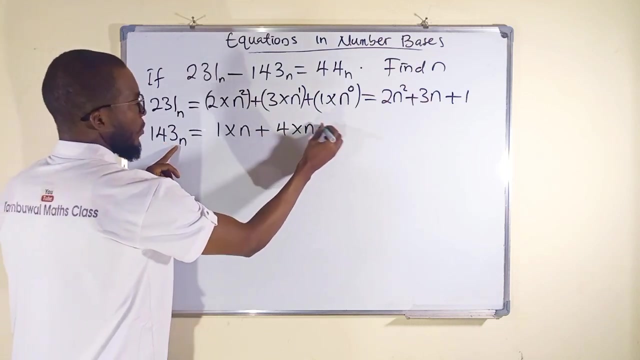 n power 1 is n times 3 is 3 n. And lastly, n power 0 is 1 times 1 is still 1.. Then we take the second one: 1, 4, 3 base n equals 1 times n plus 4 times n plus 3 times n. 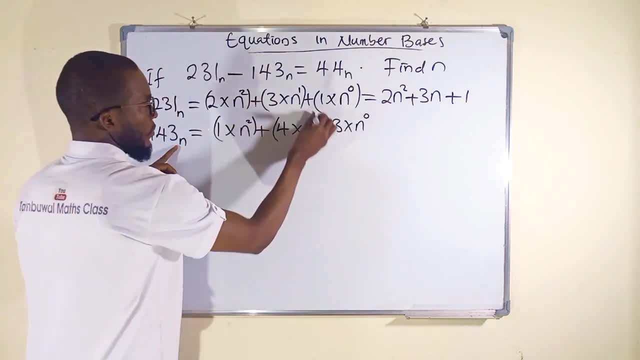 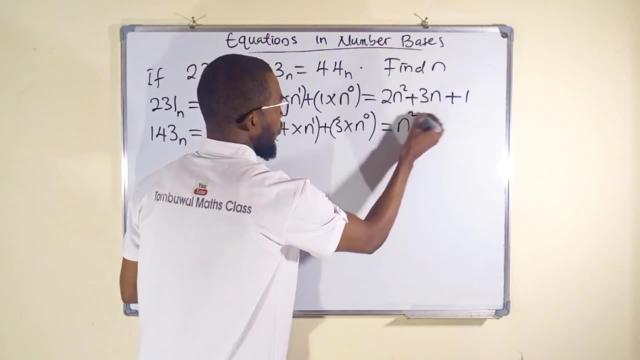 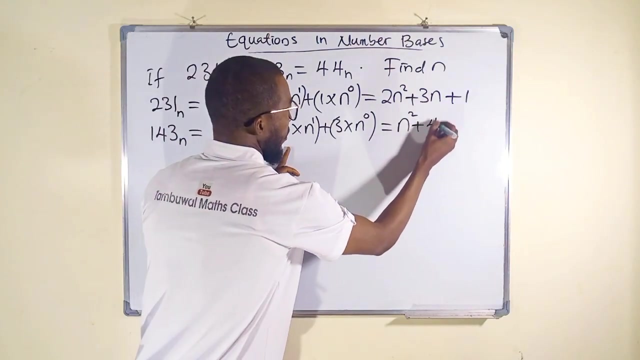 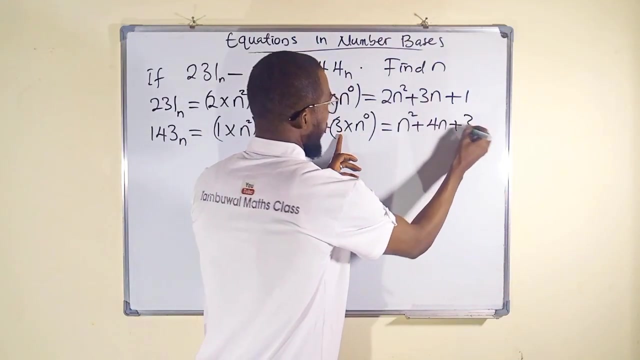 1, 2.. n squared times 1 is still n. squared n power 1 times 4 is 4n. Then n power 0 times 3 is 3, because n power 0 is 1.. Okay, Then the last one. we have 44.. 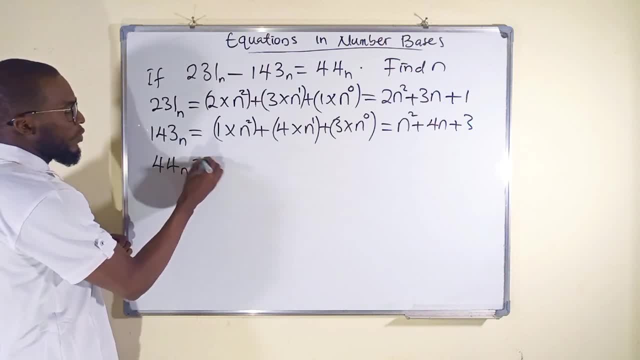 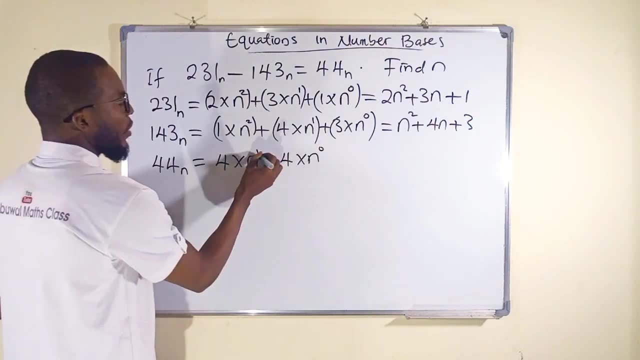 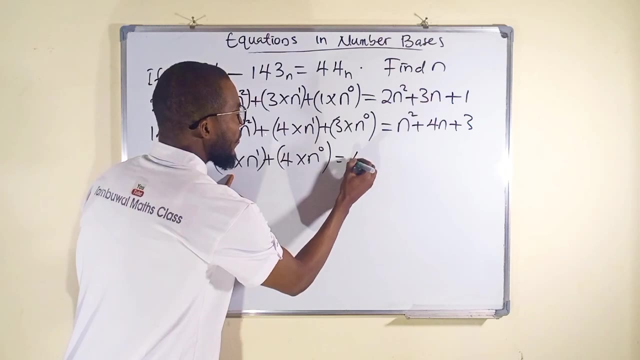 44 base n will be equal to 4 times n. plus 4 times n, We have 0 and 1.. n power 1 is n times 4 is equal to 4n. n power 0 is 1 times 4 is 4.. 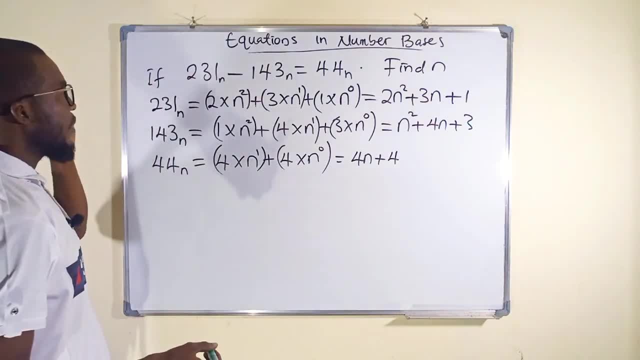 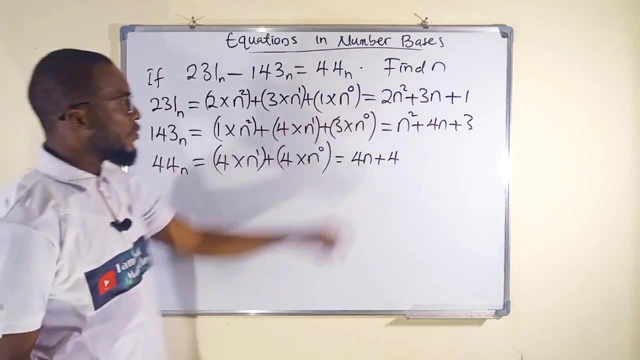 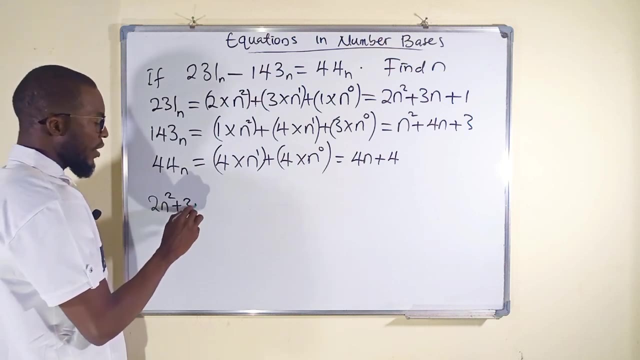 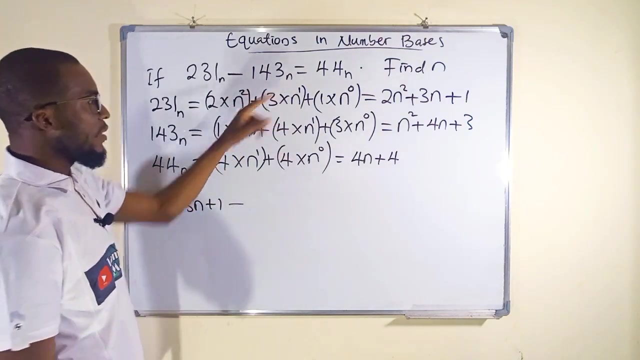 Now we can substitute back into the main equation. For this one we have 231. base n is equal to this. So we write that one 2n power 2 plus 3n plus 1.. We subtract 143 base n is now equal to n squared plus 4n plus 3.. 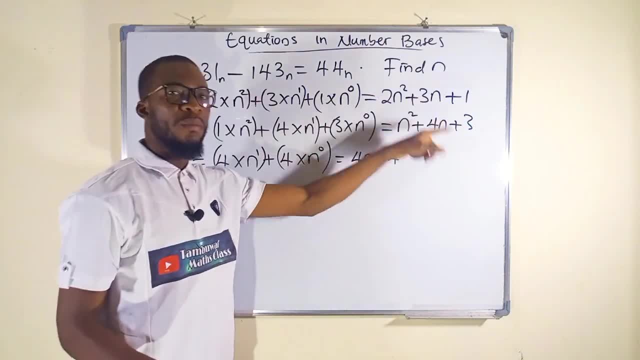 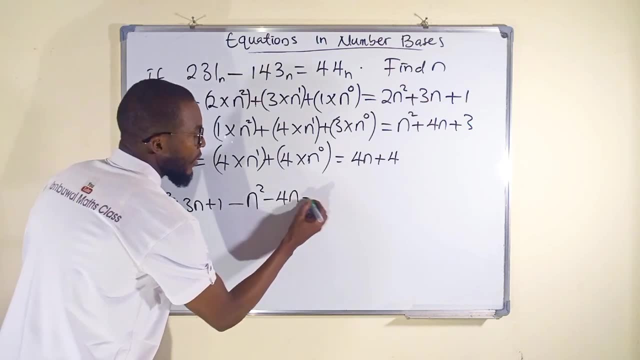 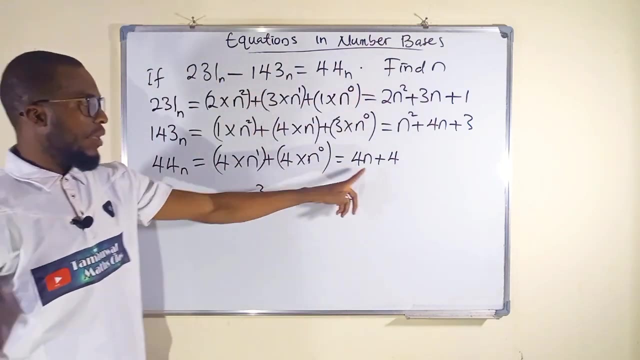 But this minus will affect each number there or each term. So minus n squared minus 4n, then minus 3.. They say this is equal to 44 in base n, And 44 in base n is now 4n plus 4.. 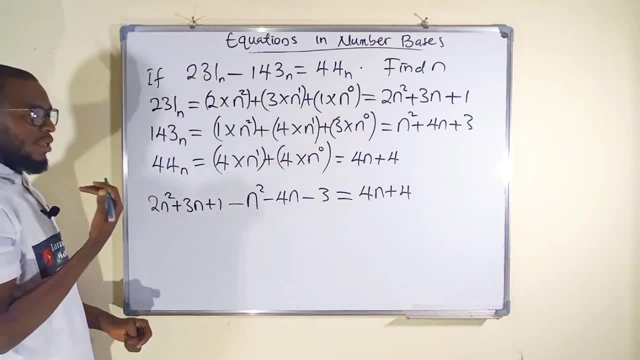 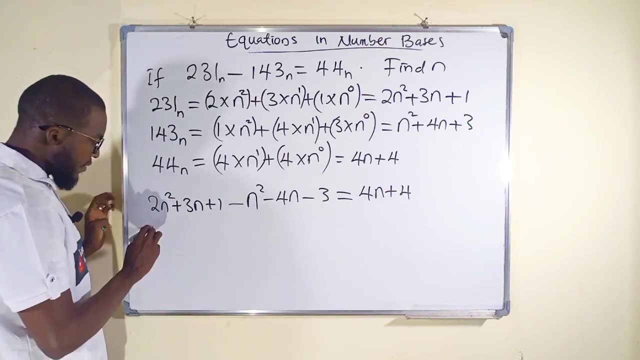 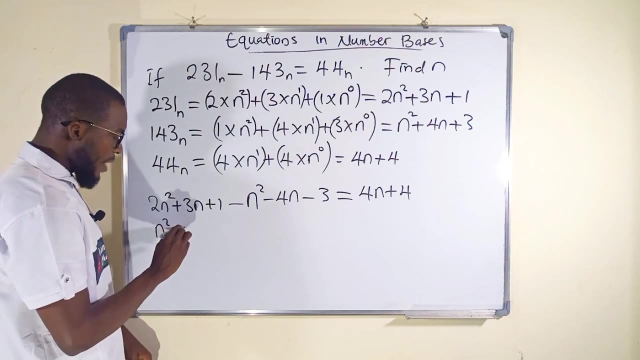 Now we want to ensure we have everything to the left, But let us first of all simplify the left. 2n squared minus n squared is single n. Single n squared: 3n minus 4n is minus n. 1 minus 3 is minus 2.. 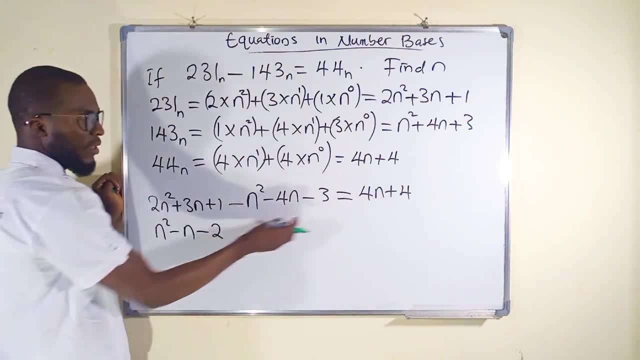 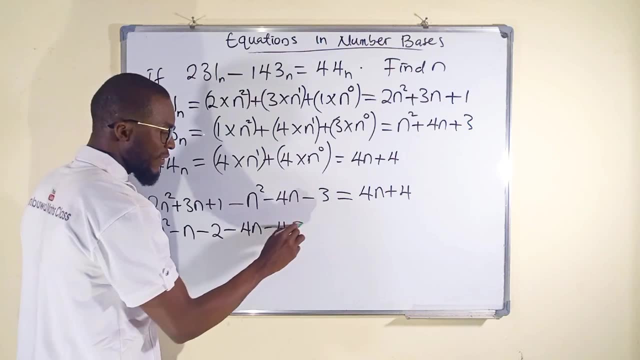 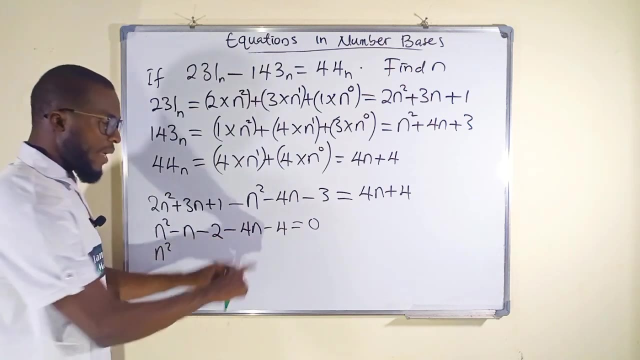 So we want to bring this one inside. If they come in, they change their sign: Minus 4n, minus 4.. The whole of this equal to 0.. n squared minus n minus 4n, 4n is minus 5n. 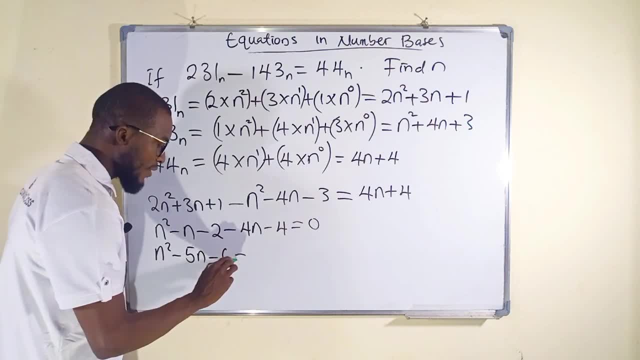 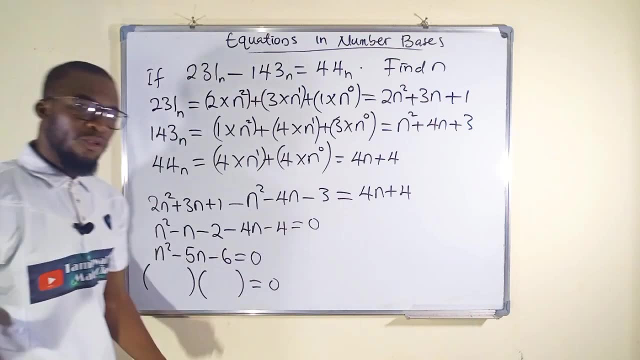 Minus 2, minus 4 is minus 6.. The whole of this equal to 0.. We can solve this quadratic equation by factorization. We are going to think of two numbers, Which one? we multiply them together, we get negative 6.. 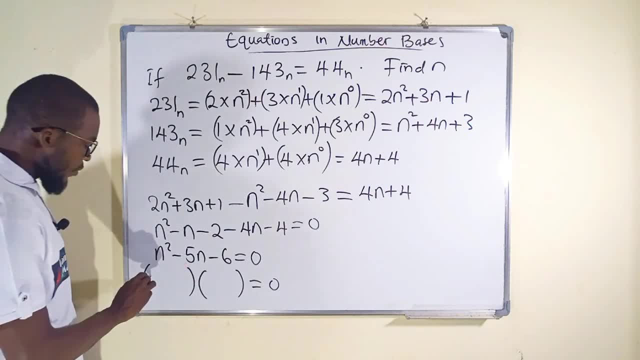 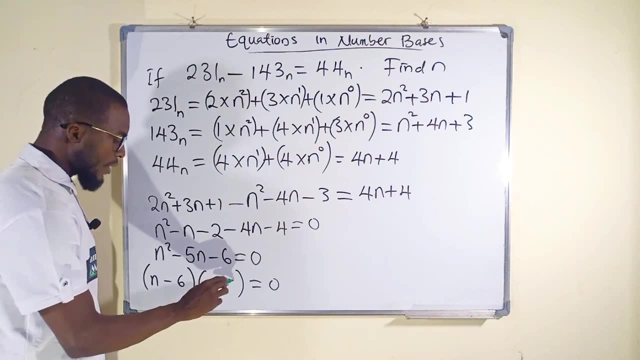 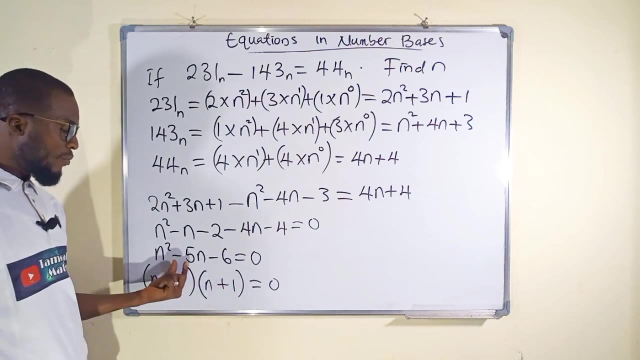 And when added up together, we get negative 5.. So we have n here. We have n here. Therefore, the numbers will be minus 6. And plus 1. Because this times this is minus 6. And this plus this is minus 5.. 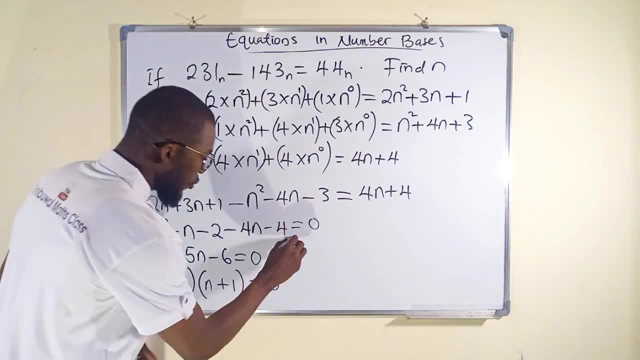 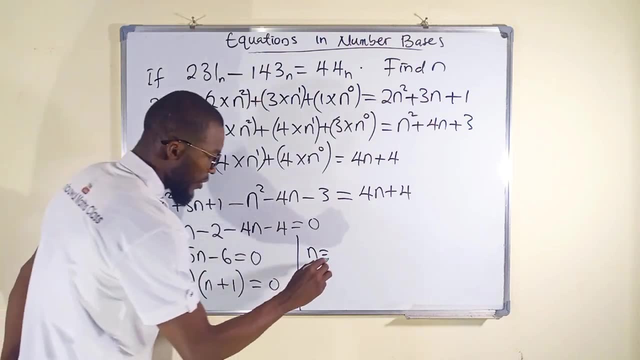 If you set each of these factors to be equal to 0, the first factor, n, will be equal to: if negative 6 crosses over equality sign, it becomes positive 6.. And the other one, if positive 1 crosses over equality sign. 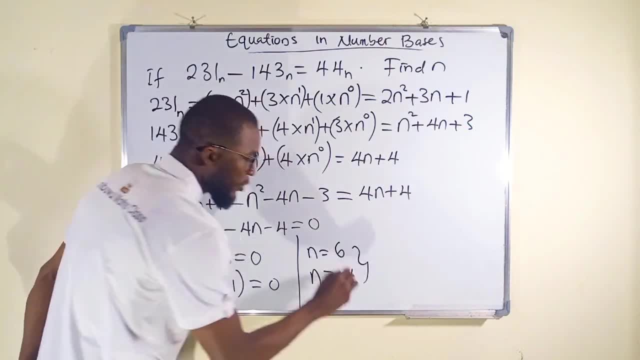 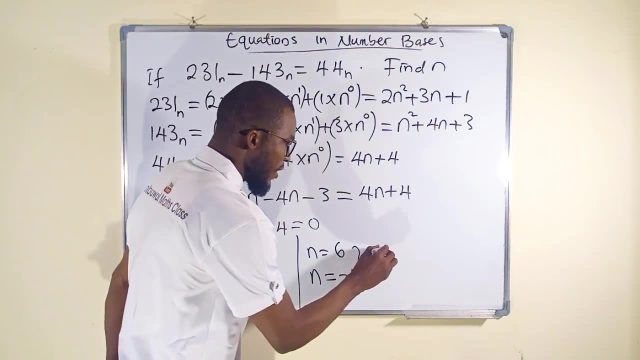 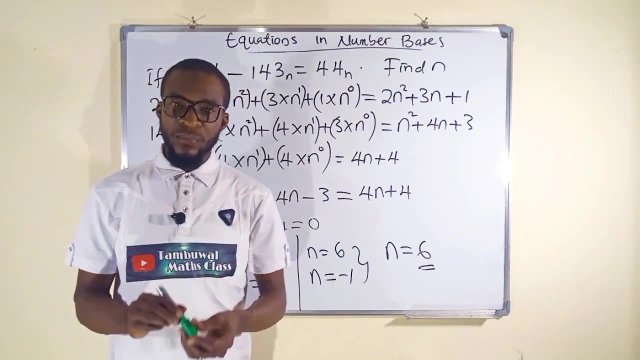 it becomes negative, So we have negative 1.. These are the two possible solutions. But remember, n is base And we do not have negative base And therefore we see n equals 6 as our answer. Now let us look onto the next question. 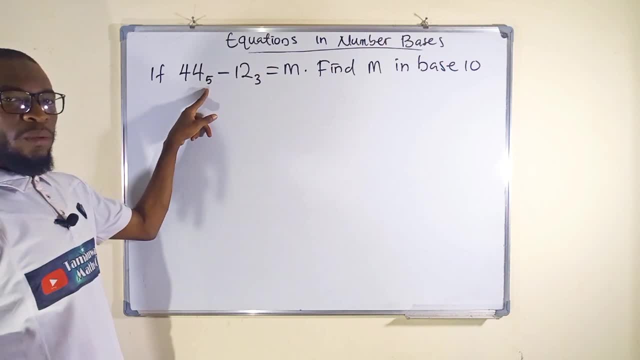 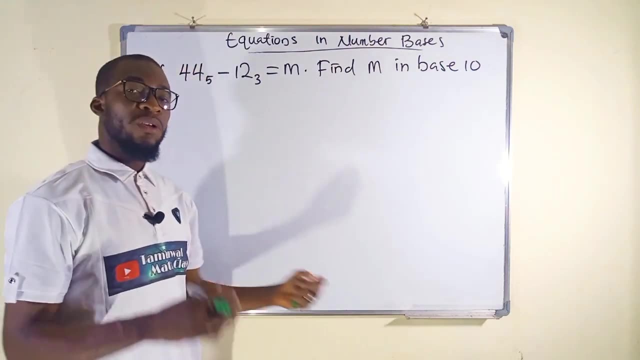 Our third question says: if 4 to 4 in base 5 minus 12 in base 3 equals m, we are asked to find this m in base 10.. Since we are looking for m in base 10, we are free to convert each of these times. 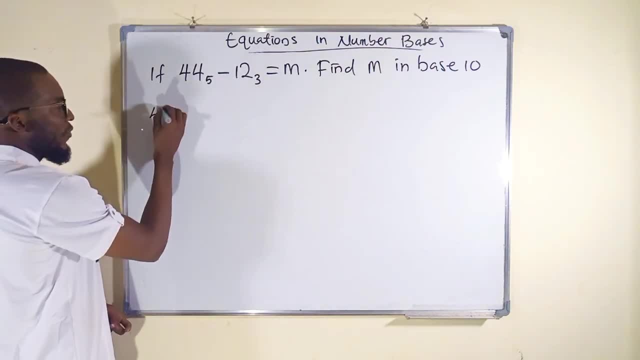 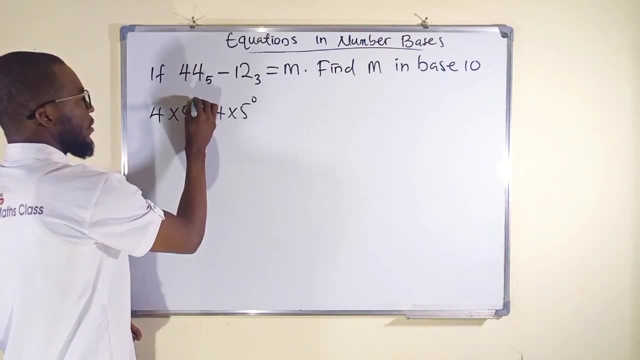 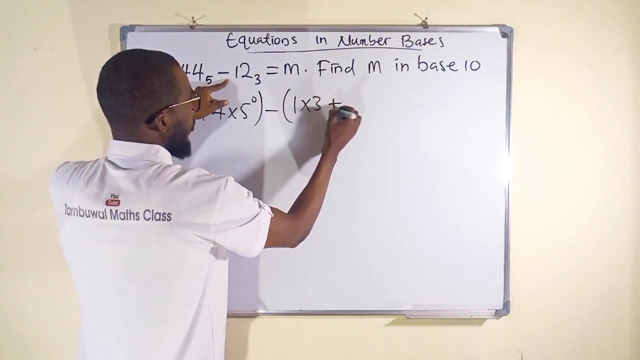 to base 10.. The first one we have 4 to 4. This is 4 times 5 plus 4 times 5.. 0 and 1. We subtract this one, We have 1 times 3 plus 2 times 3.. 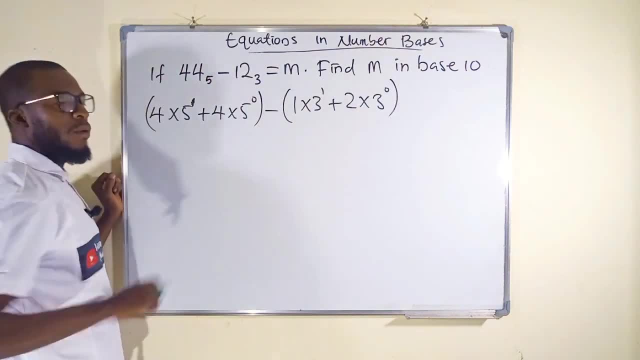 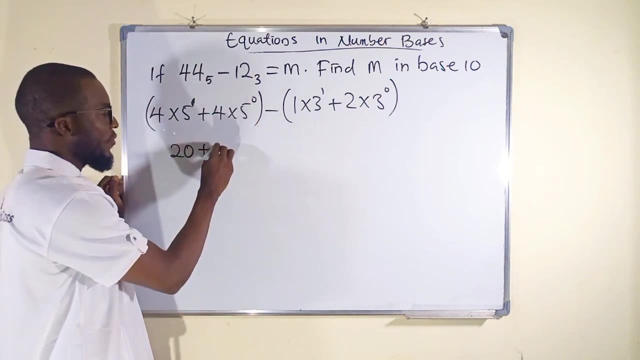 0 and 1.. We simplify: 5 power 1 is 5 times 2 is 20.. 5 power 0 is 1 times 4 is 4.. Minus 3: power 1 is 3 times 1 is 3.. 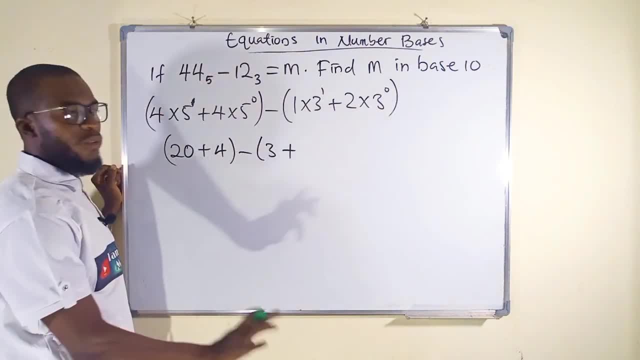 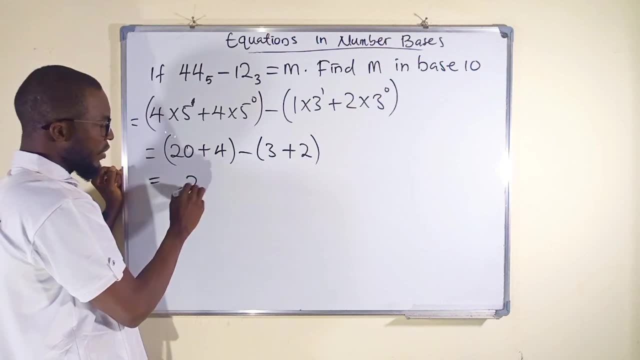 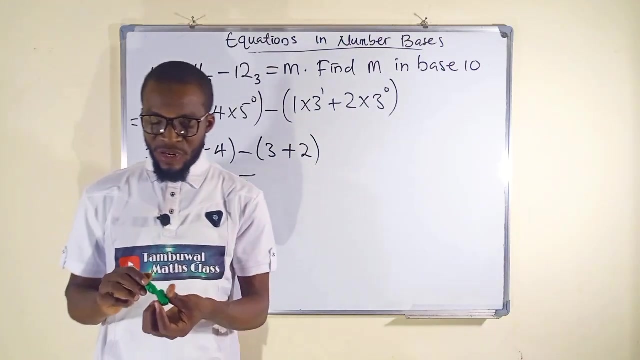 Plus 3, power 0 is 1 times 2 is 2.. This is equal to 24 minus 5.. And this is equal to 19,, which is the value of m, And it is in base 10.. Let us look onto the next question. 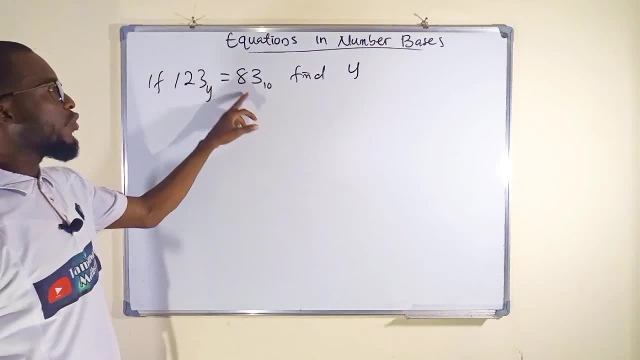 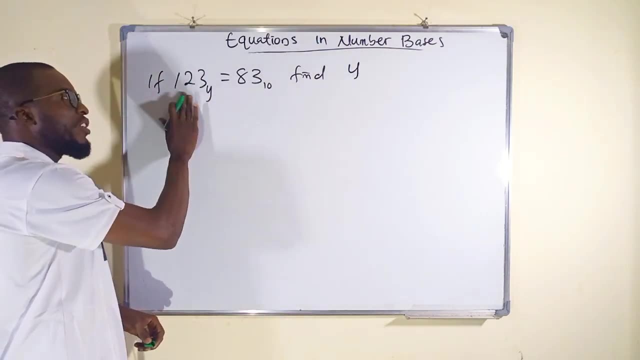 Our fourth question says: if 123 in base y equals 83 in base 10, we are asked to find y. Since 83 is in base 10, we are free to change this one to base 10 and equate them together. 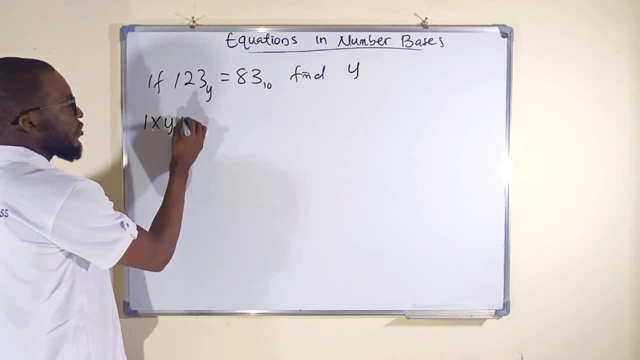 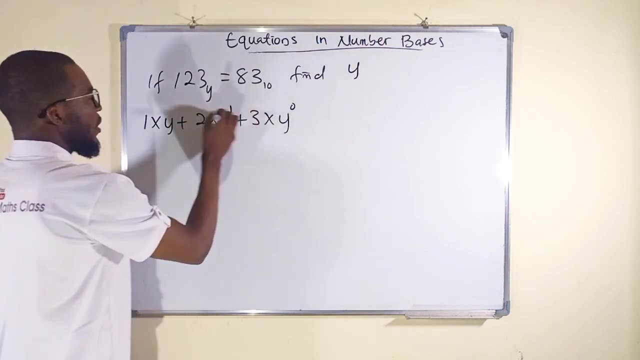 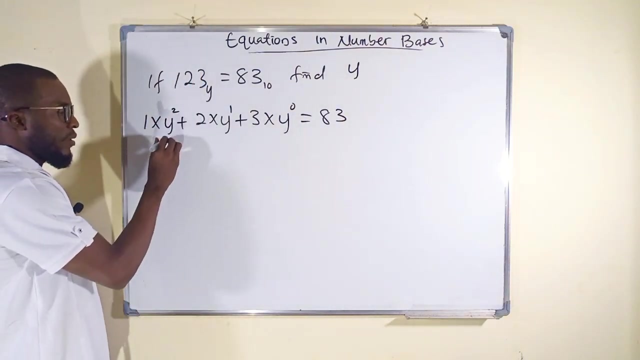 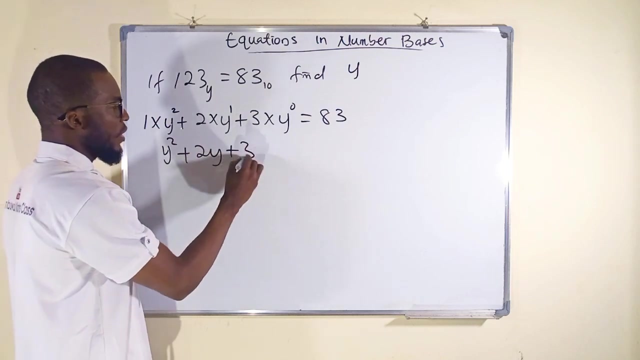 This becomes 1 times y plus 2 times y plus 3 times y, 0,, 1, and 2.. The whole of this equals 283. as required. This is y squared plus this is 2y. y to the power of 0 is 1 times 3 is 3.. 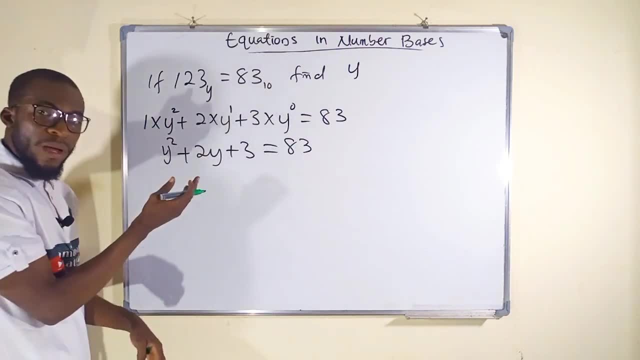 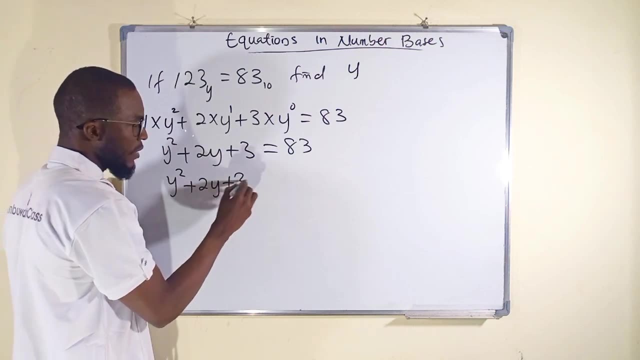 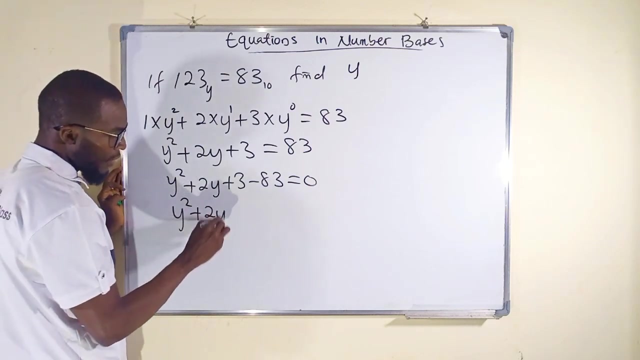 This is equal to 83.. We can bring 83 backward and it becomes negative. This is y squared plus 2y plus 3, then minus 83. The whole of this equals 0.. y squared plus 2y plus 3 minus 83 is negative 80.. 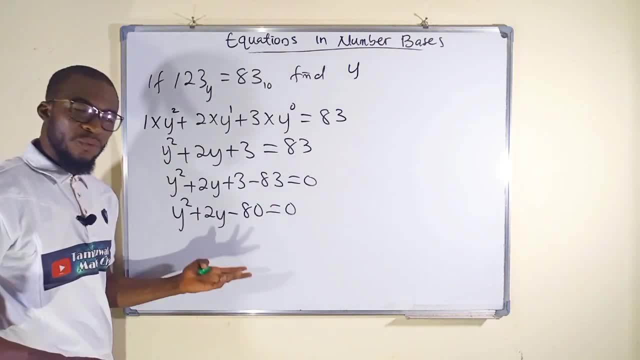 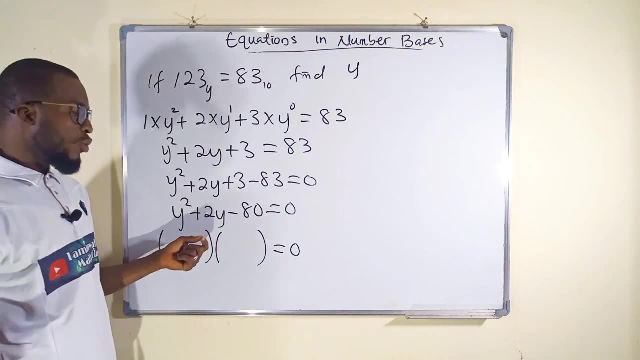 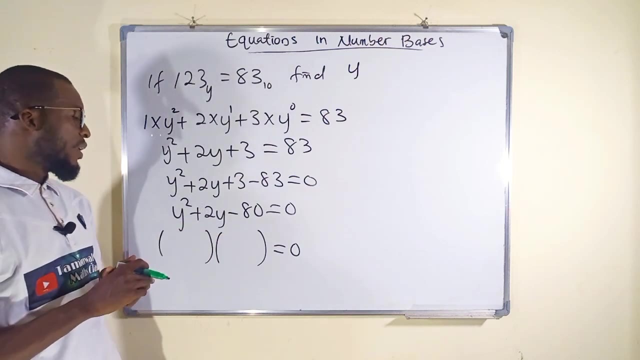 The whole of this equals 0.. We have now formed a quadratic equation which we can solve by factorization. We are going to think of two numbers which, when we multiply them together, we get negative 80. And when we add them together, we get positive 2.. 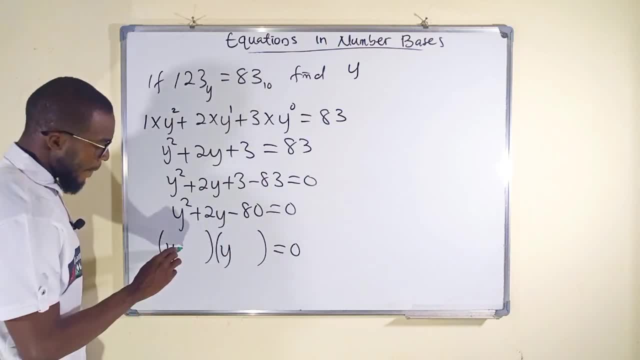 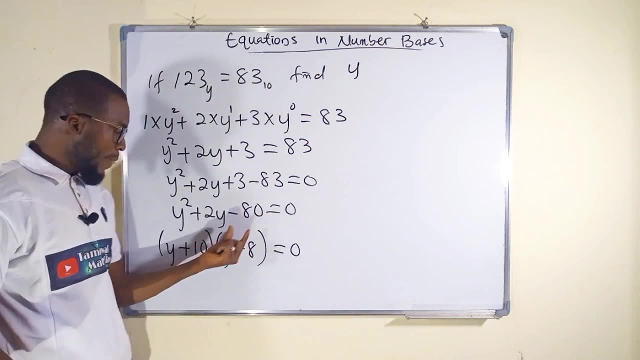 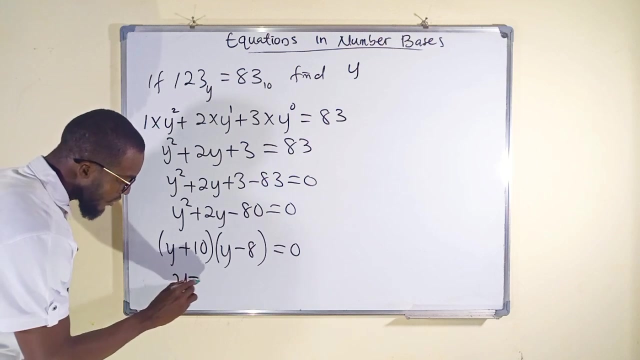 The numbers are positive 10 and negative 8, because this time this is negative 80 and this minus this will give us 2.. If you set this one to be equal to 0, you obtain y equals negative 10.. Or if you set this to be 0: 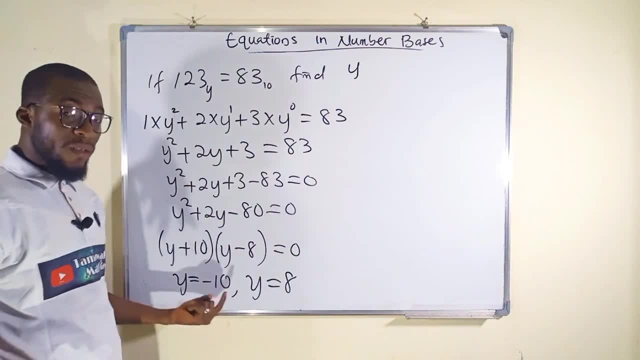 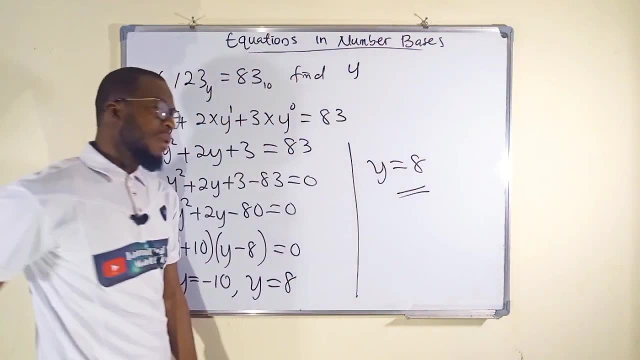 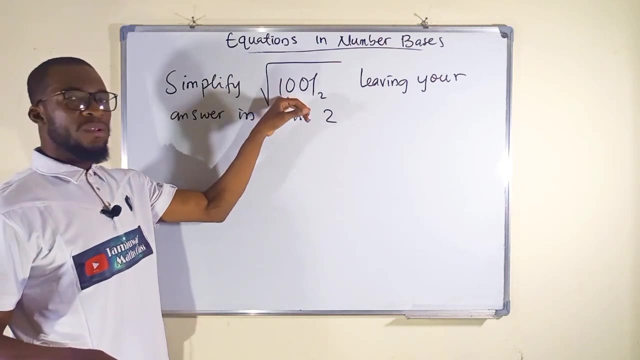 you get: y equals positive 8.. Remember, y is our base, so we can't take negative value. And finally, y equals 8.. Let us take another one. So here is our last question. We are asked to simplify the square root of a number in base 2.. 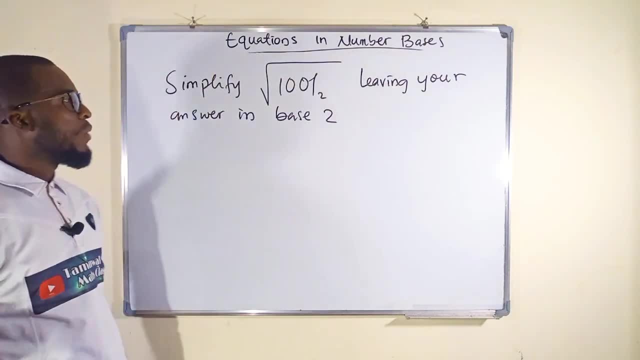 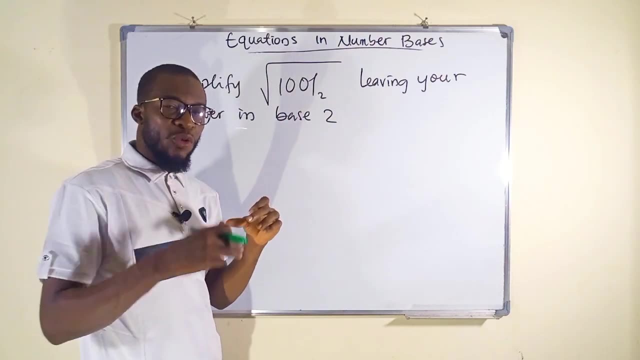 And we want to even leave the answer in base 2.. We know it is very difficult for us to take the square root of a number in base 2. But we are free to convert that number into base 10.. Take the square root and reconvert it back into base 2.. 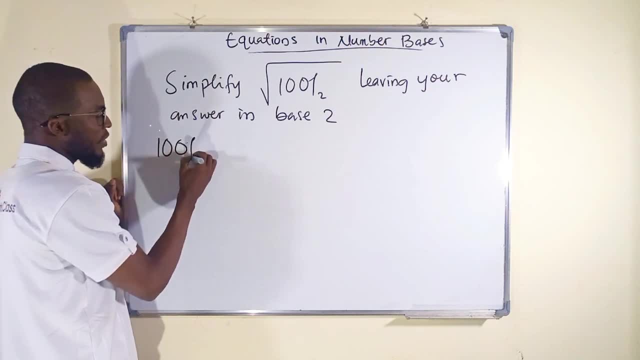 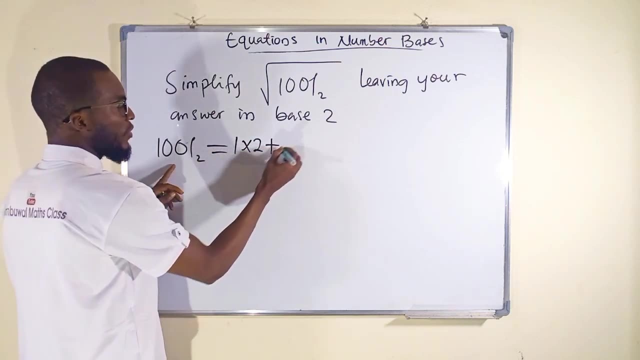 Let us do that. We have 1001 in base 2.. We want to change it to base 10.. We take the first digit, 1. We multiply by the base 2. Plus 0 times 2. Plus 0 times 2..